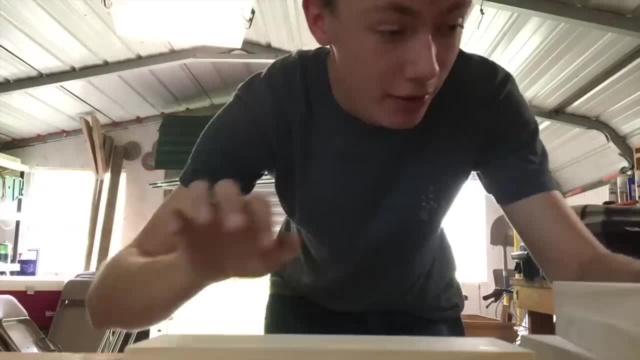 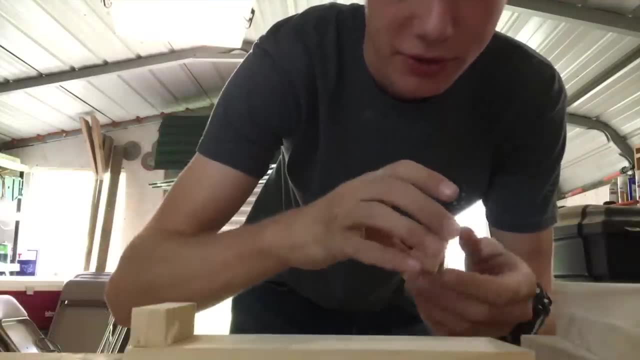 All I'm going to do is just lay one out, take two of the legs. I tend to put the rough side down, so that way that's not the one that's showing, and that's it. All I got to do is either glue it. 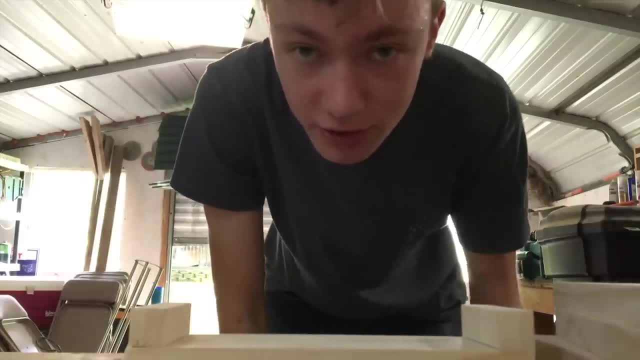 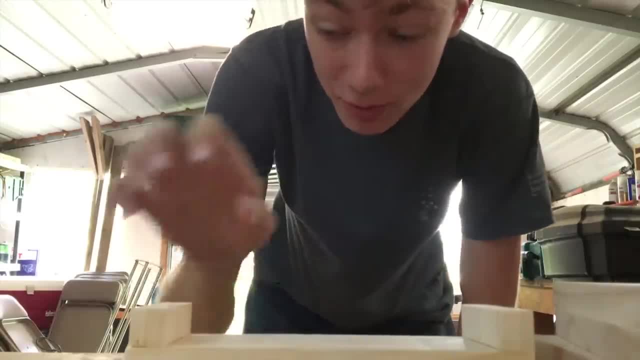 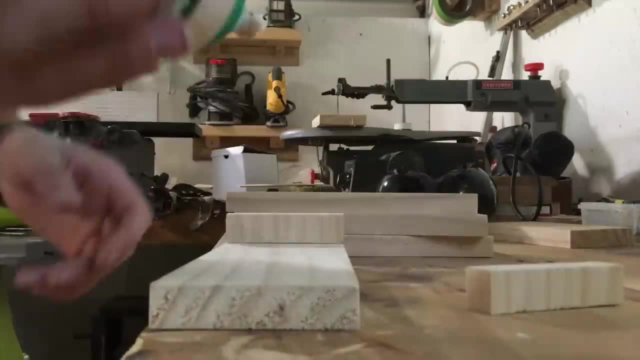 I'm going to try to glue it and brad nail it from the bottom down, since nobody's going to be seeing this anyway. So all I'm going to do is use some Titebond 3.. It's my favorite glue. I've tried, you know, the other brands. 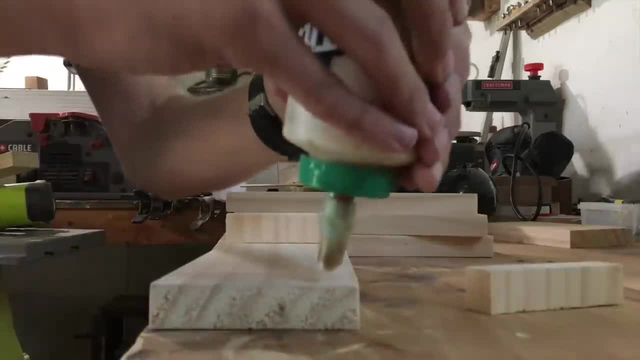 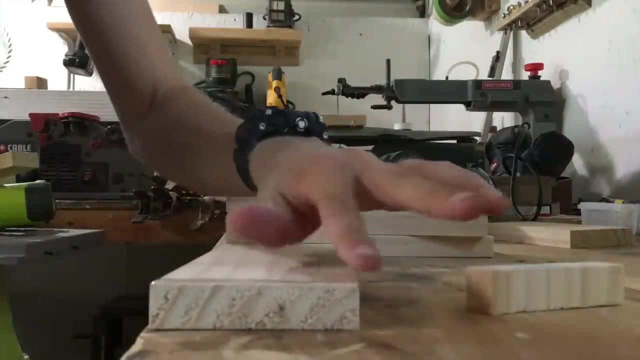 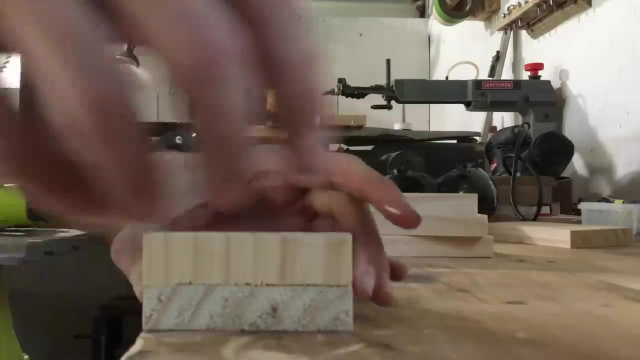 It just doesn't seem to work as well. So all I'm going to do is just apply just a thin layer, kind of mush it in with my finger just to kind of spread it out, and then just attach it, And then you can either clamp it with 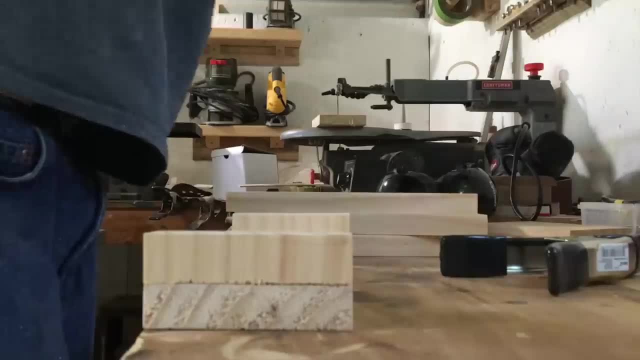 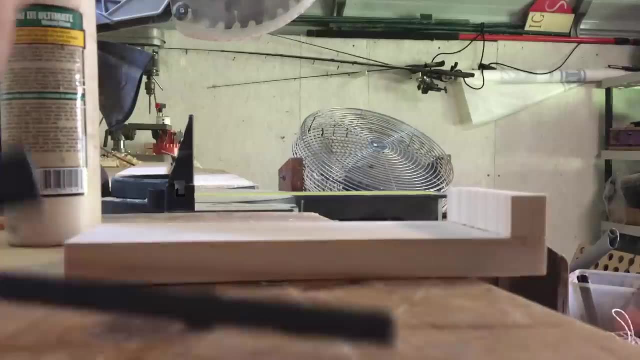 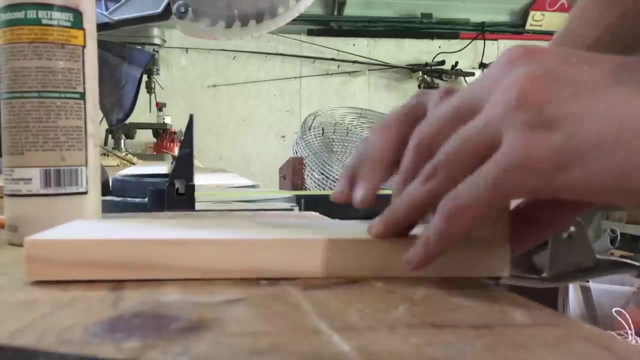 a spring clamp, or I have these trigger clamps as well, So either one will work. I would recommend, if you do have super glue or an accelerator, to use those. I have been doing this the whole entire time, but it's just annoying having to wait for the glue to dry. 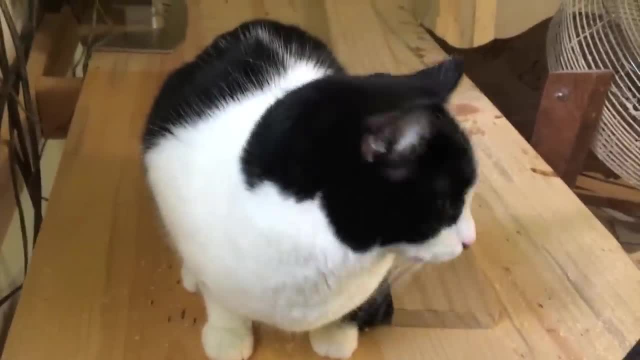 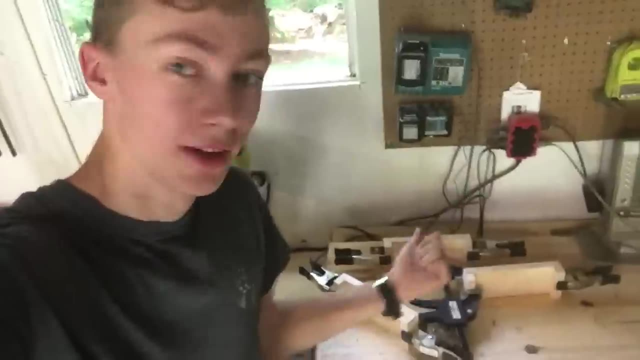 Hey Loosh. So, as you can see, I already got three done. I mean, it's super simple. As long as you got the clamps, you got the glue, it works perfect. Now, over here, I'm going to do one more. 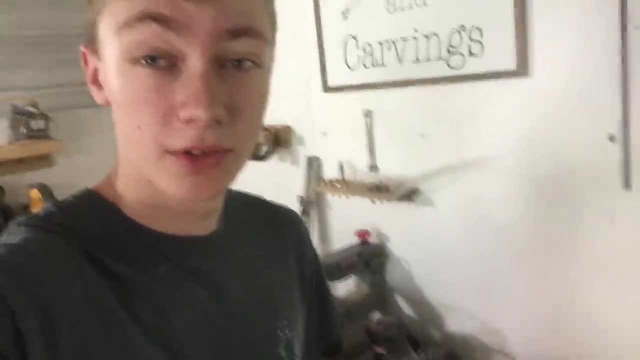 I'm going to do one more, but this time I'm going to try to do it with brad nails, Glue it and then add some brad nails so I don't have to have clamps. The only issue that I'm having with it is: I'm kind of afraid because I'm shooting, you know. 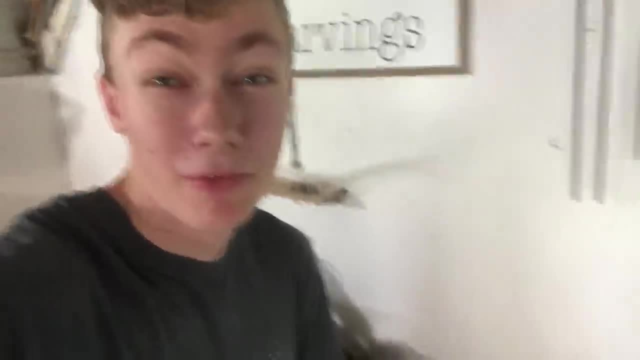 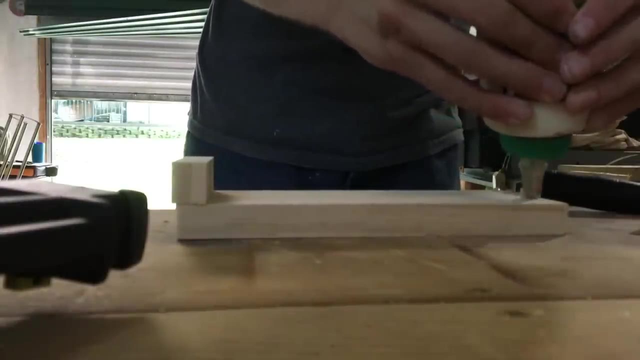 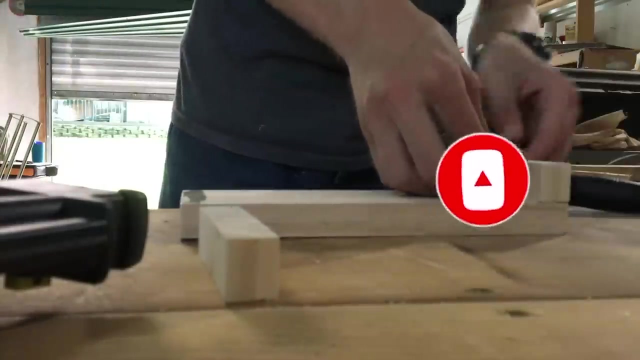 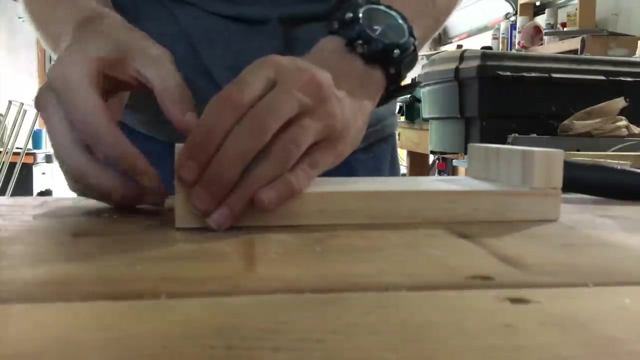 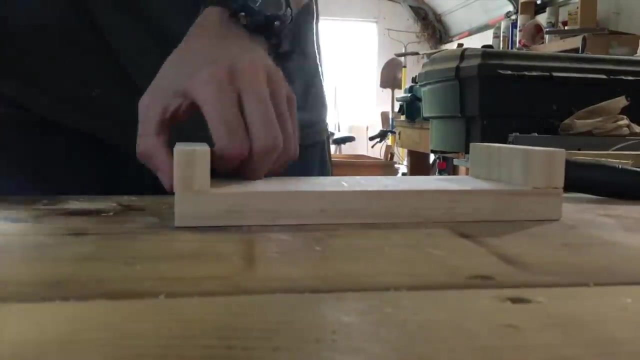 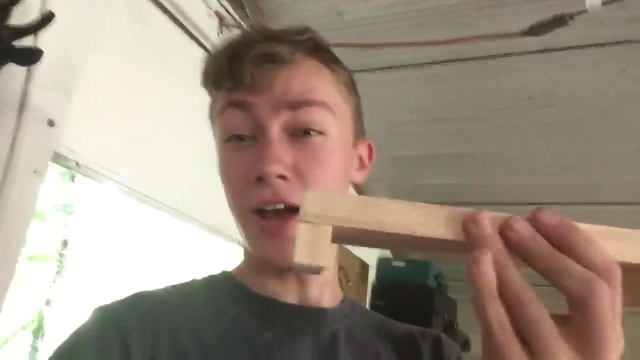 on the top with the grain going in. I'm afraid it's going to split, but we'll try it. So here it is. Hello guys, I just revolutionized my way of woodworking this whole entire time, So I'm going to do one more. 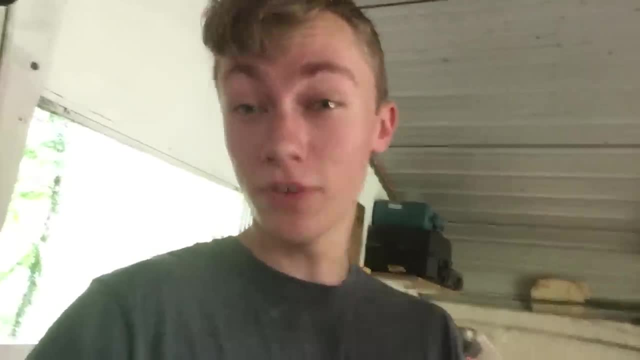 I've been gluing it, I've been waiting 24 hours for it to cure, and then I'll move on to the next step. Look how easy that was: No splits, No, nothing, And I can't even be able to see it. 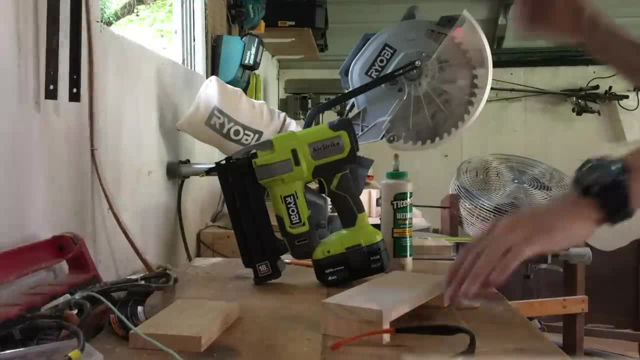 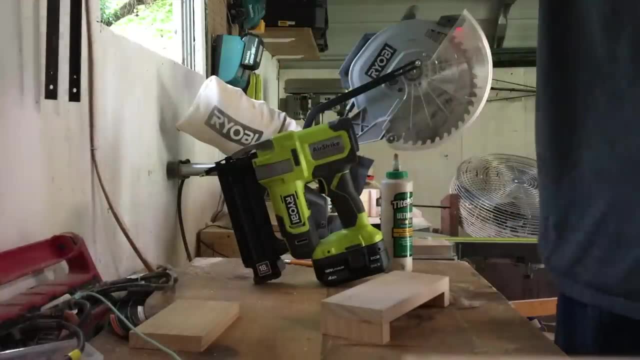 And, yes, make sure you have a mask, safety goggles and earmuffs when woodworking. They all have their own purpose and I can't tell you how many times I've went without safety glasses. No metal or wood has launched into my eye. 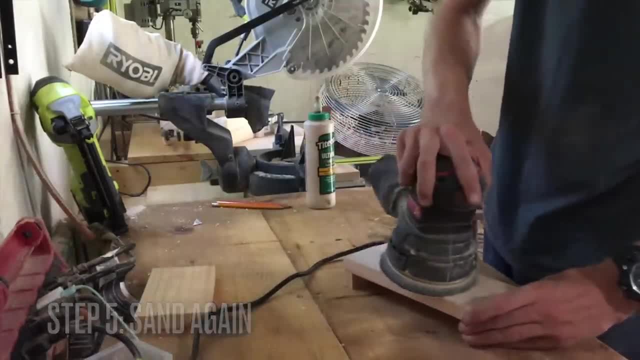 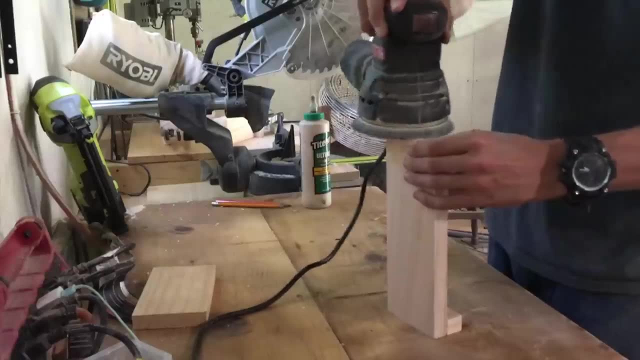 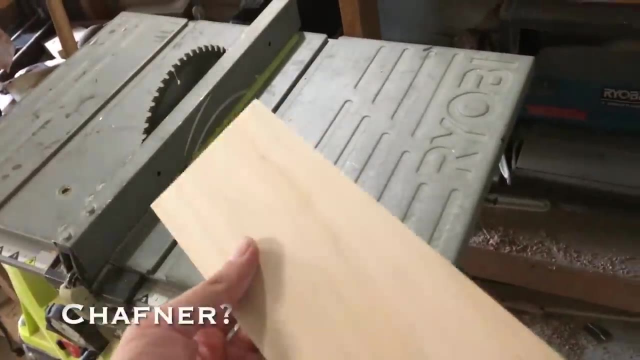 Step five is just sanding again, Just making sure there's no furs, making sure there's nothing sticking up, Just to make sure we're all nice and smooth. Okay, so this next step I've kind of had to rig, because I don't have a chafner bit- the 45 degree one. 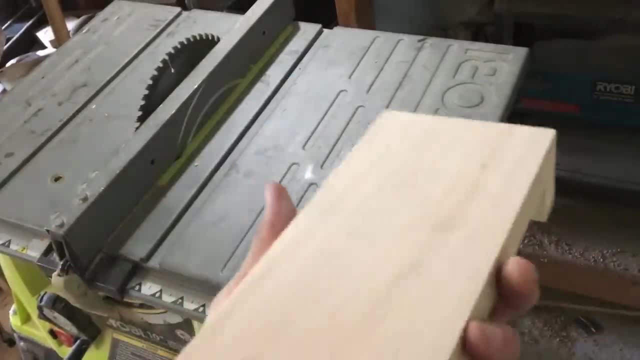 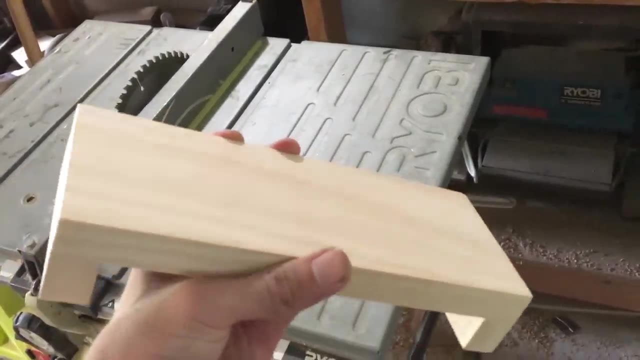 So I'm just going to have to do it on the table saw. This is just going to kind of give it. you could leave it like this and it looks fine, Just stain it and clear it. But I like to add just a little bit of a more decorative look to it. 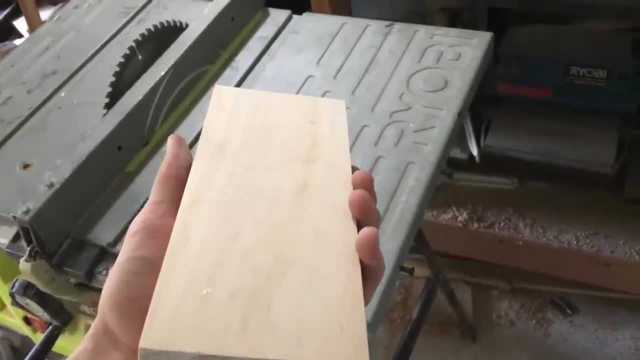 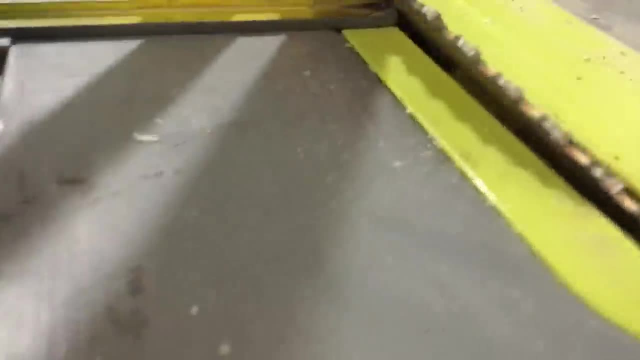 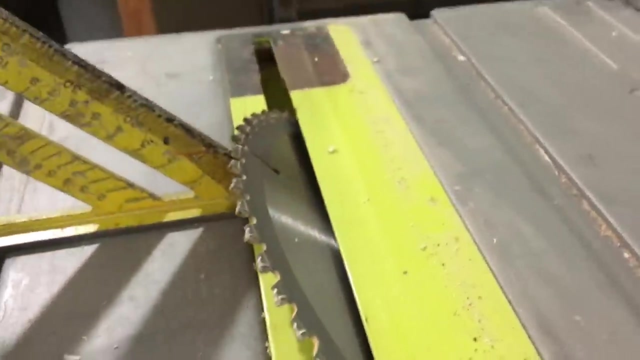 So let's move to the table saw. Put your saw blade at 45 degrees Re-angle. This doesn't have to be exactly 45 degrees, because it's just going around the edges, sort of like what a router bit would do. 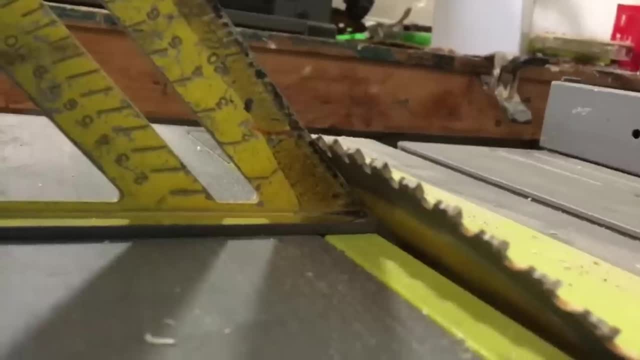 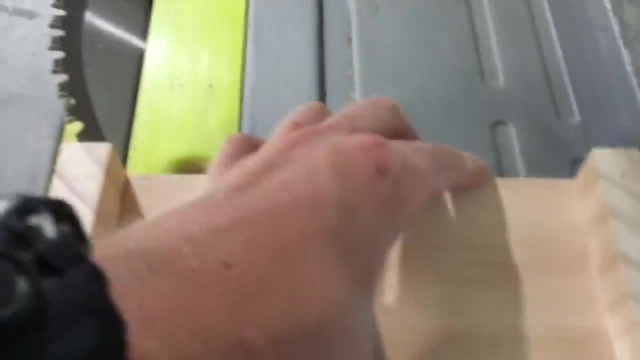 So it doesn't have to be exactly, but just to show. if you wanted to make it exactly, just use a speed square And you can tell it's 45.. So you want to move your table saw fence just enough to where it doesn't cut the whole thing at 45,. 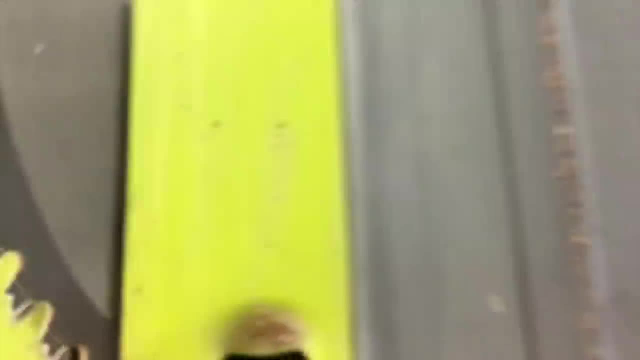 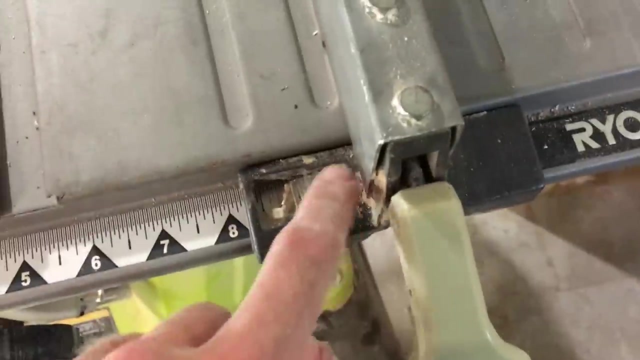 but just the tip of it into a 45 degree. So how I did this was I just memorized. just put it after the second bubble. That's how I did it. Or you can stick a piece of tape, painter's tape or something underneath it. 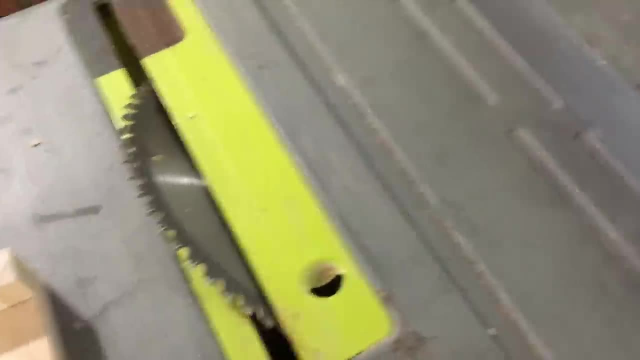 And I'll show you how to do it every time. That's just how I do it, But again, you'd use a chafing bit at 45. That would be. that would definitely be a lot faster, but I don't have one. 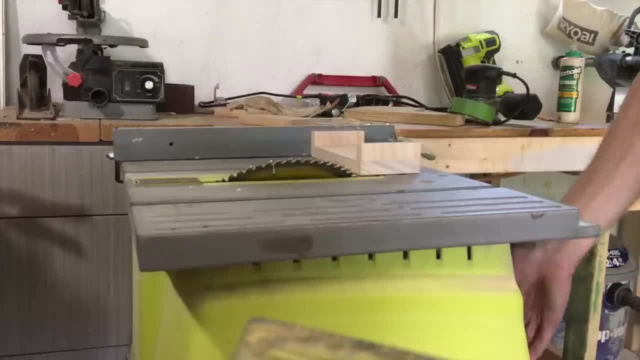 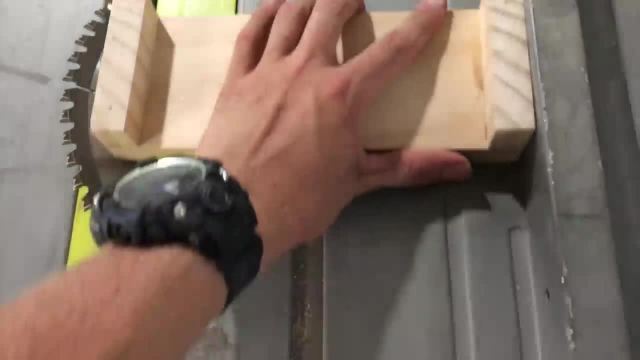 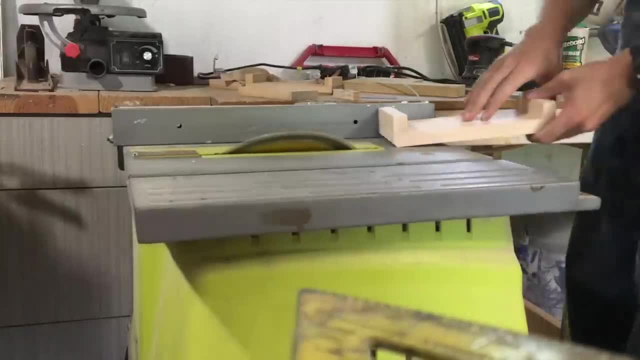 And that's how I do it on both corners, And I'm just going to do it on this side as well. If you're going to do it this way, please be mindful where your fingers are, because your fingers can get close to the blade. 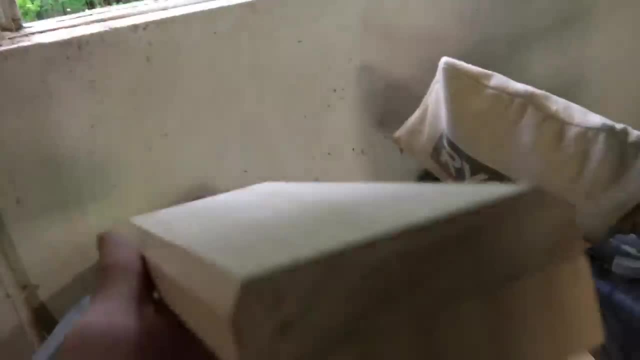 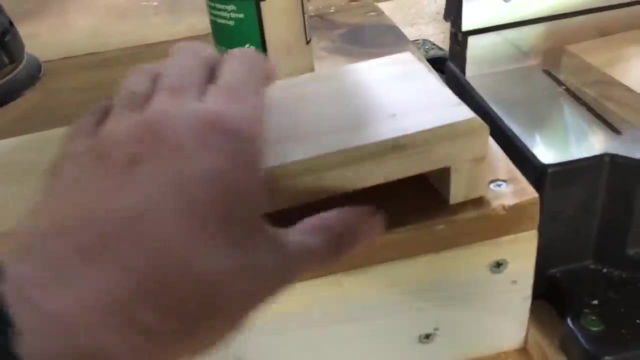 Sorry for the loud noise. It's raining outside, But anyway, as you can see, I did a 45 degree around the whole thing and it just kind of gives it just like, makes it more decorative, I think, if you wanted to, because, like here, if you don't have a tampon bit. 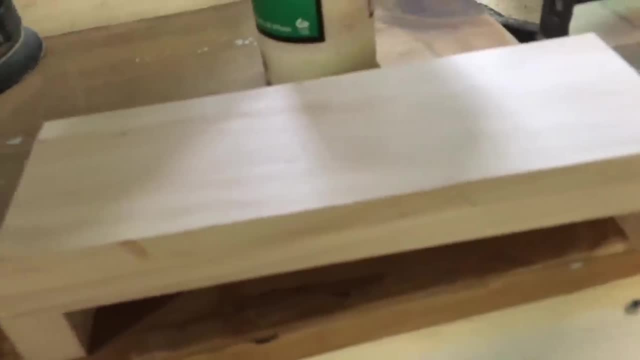 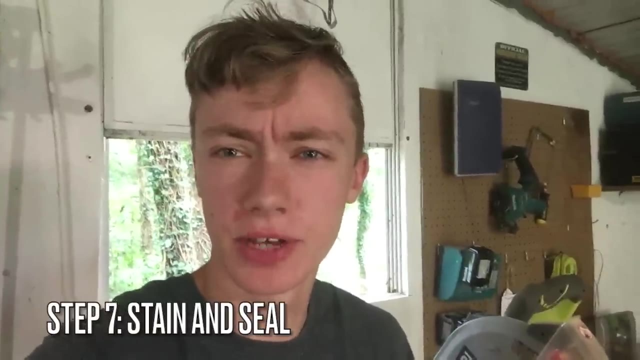 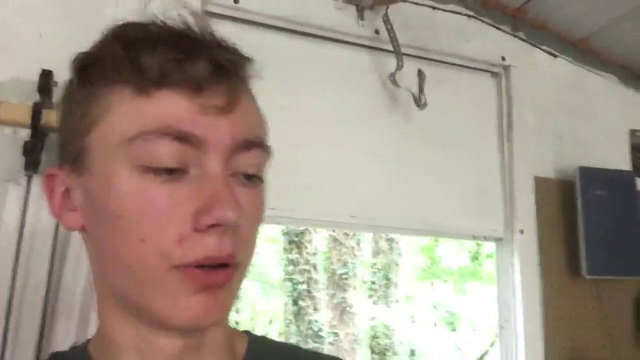 I got a little saw nick right there and I can just sand that off, So You could go with the sand and then next is just staining it. So it's good to have variety. It's kind of a good marketing thing. So what I like to do is I like to use Kona, which is a brown, and then I also do an ebony. 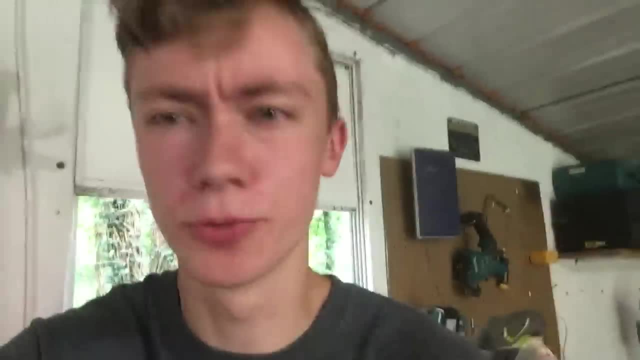 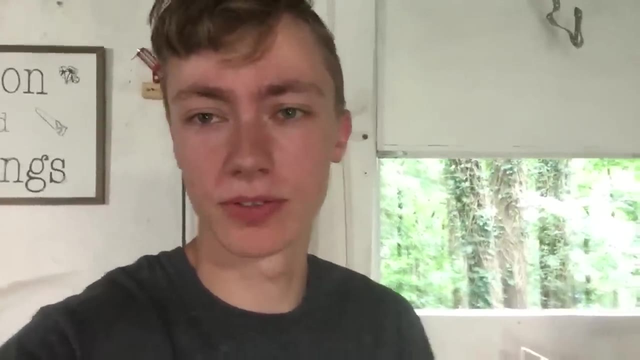 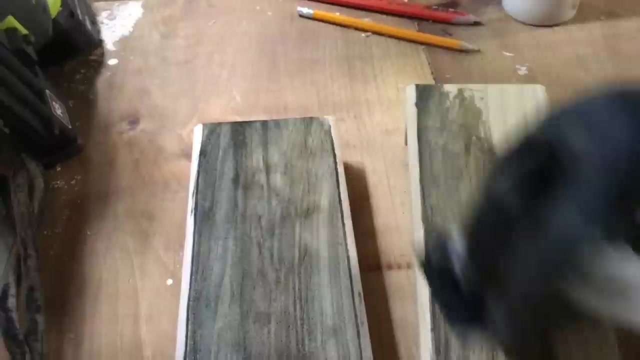 which is black, And then I also do a raw, but most people don't buy that, but it's there if they want it. But both of those sell basically the same and I've probably sold about the same amount of both. So here's your final product. 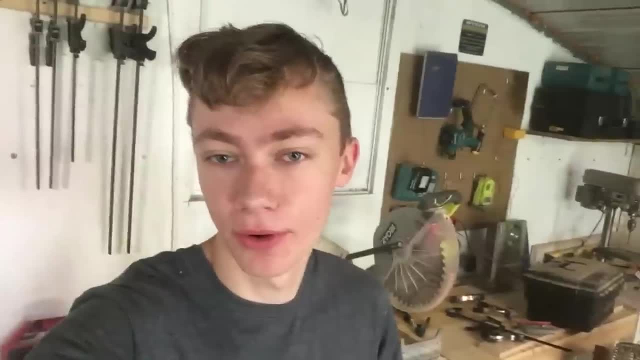 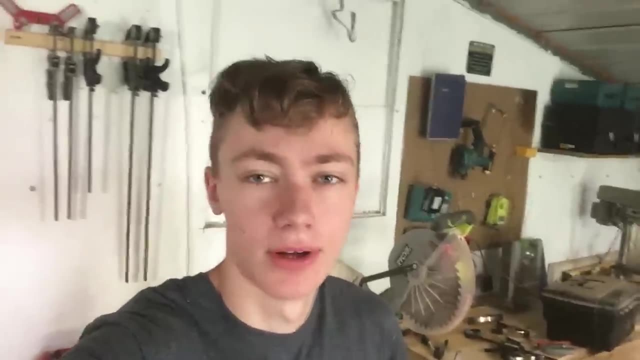 Looks very nice. Looks very nice. You can add whatever clear you want to. You could do tongue oil. You could do polyurethane wipe on poly, anything that you like. But this is it. I still haven't told you what it is yet, but I'll put some pictures and show you what it. 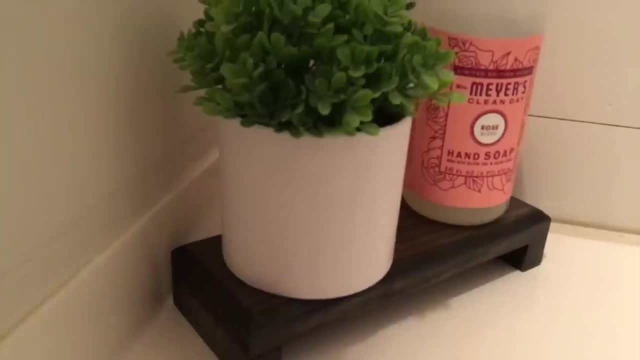 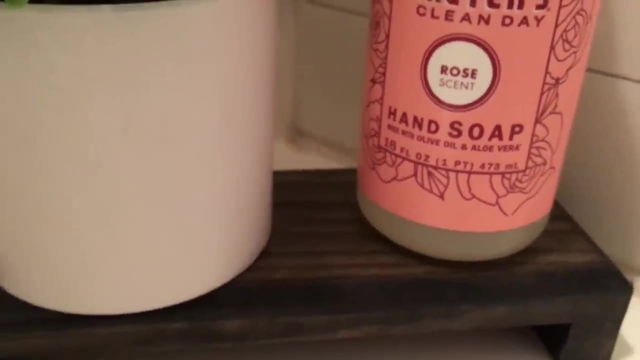 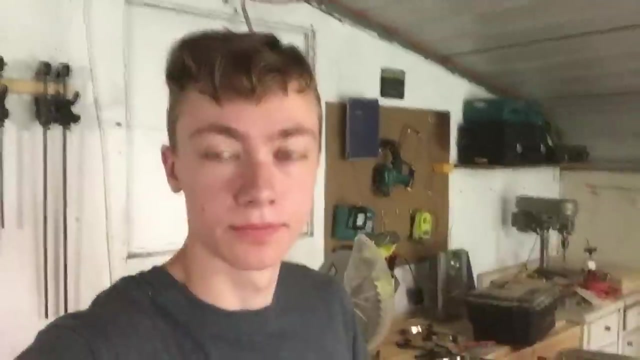 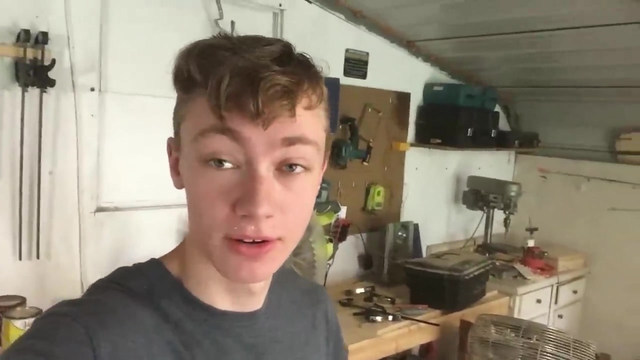 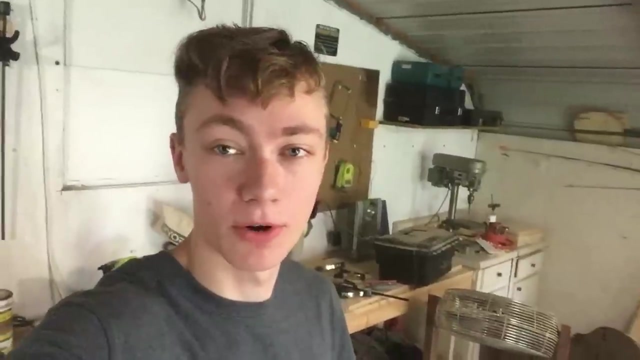 is So: yeah, something as simple as that has made me some money. I mean, it's an easy project. I sell them for $10.. You can usually on Etsy you can find them for like $15.. Since I'm using Facebook Marketplace, 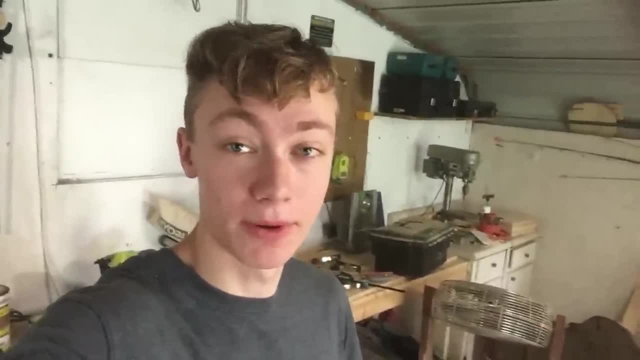 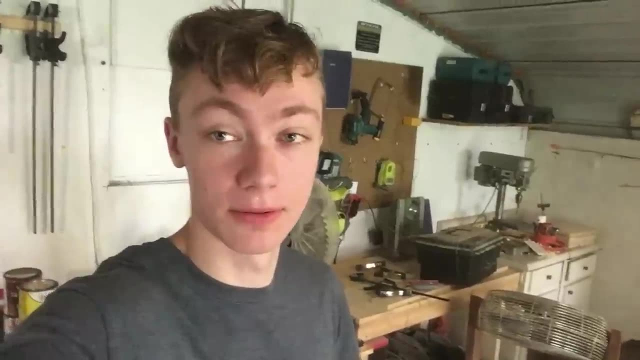 I like to bring my price down and I've sold quite a bit of them. So if you're looking at an easy way to make money, this is it. Like I said, it's done me great. So thank you guys for watching this video. 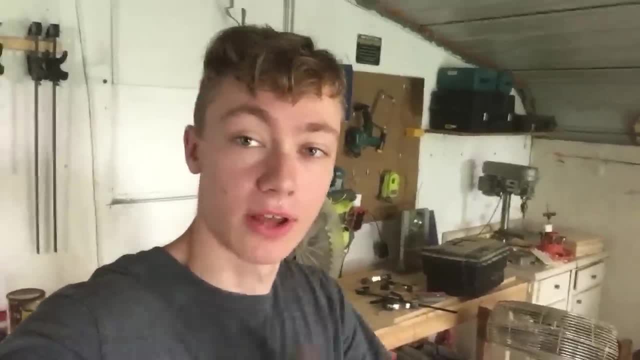 If you liked it, please hit the like button and the subscribe button and I'll catch you in the next video.